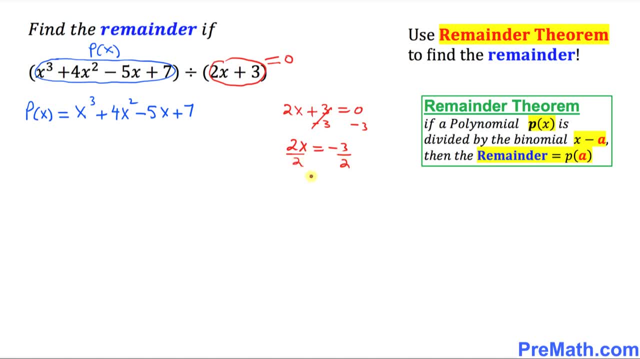 divide both sides by 2.. So x turns out to be negative 3 over 2.. So now we know that we got x equal to negative 3 over 2.. So whatever this value is, wherever you are, you can find the denominator. 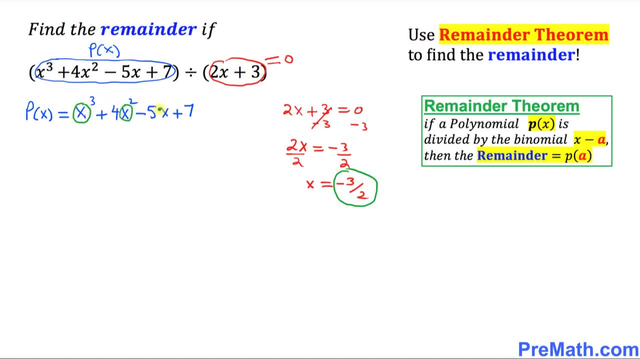 Wherever you see x variable, we are going to replace that value. So so this is going to simply become p of negative 3 over 2 equals to. So wherever you see x, replace it by negative 3 over 2.. This is power 3 plus 4 times negative 3 over 2.. 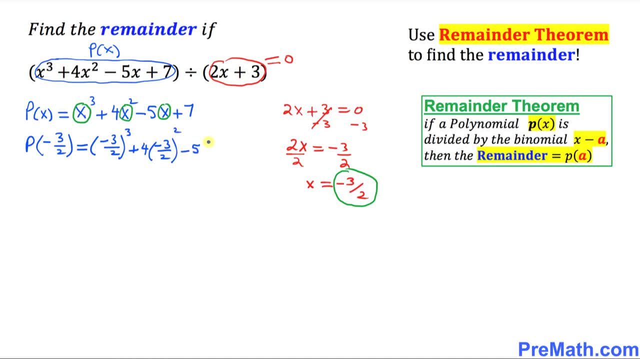 2 minus 5 times negative: 3 over 2 plus 7.. So let's simplify, furthermore, So we're going to take care of this exponent. So negative 3 power 3, since the power is r. So we're going to keep the negative. 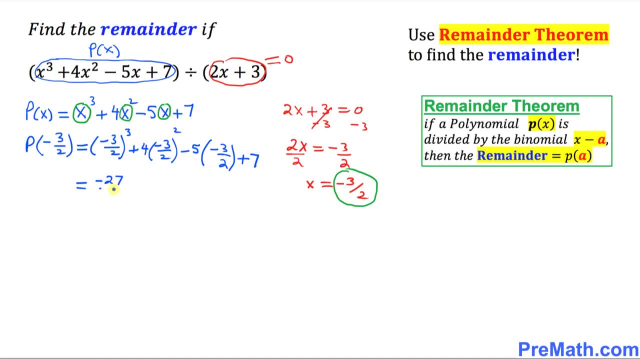 sign. So it's going to become negative: 27 divided by 2 power 3 is going to be 8.. And here, plus 4 times negative, 3 over 2 square is going to become 9 over 4.. And here that is negative and negative become positive: 15 over 2 plus 7.. We are: 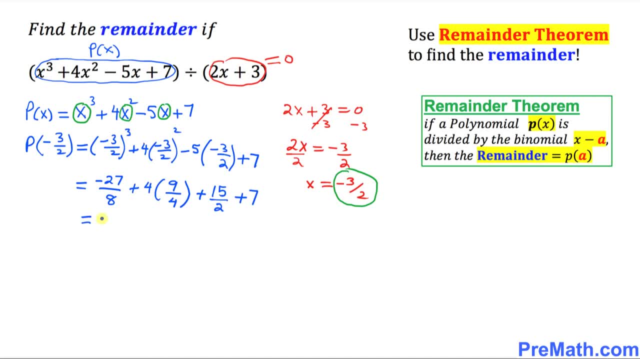 not finished yet, Let's go. furthermore, Negative 27 over 8, and here you can see this: 4 and 4, they are gone. So we simply ended up with plus 9 plus 15 over 2 plus 7.. So here you can see. 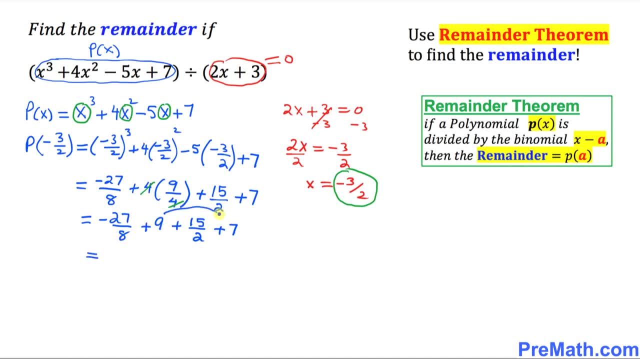 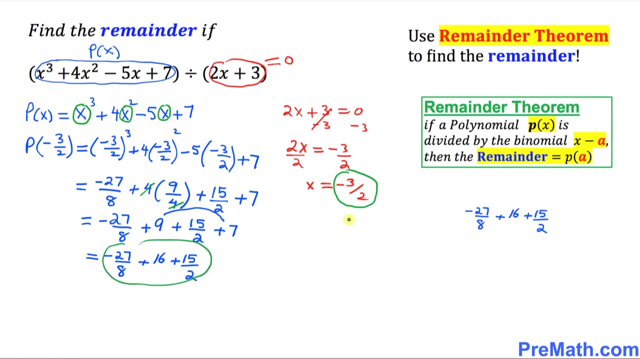 this one. I can write this one. See this: 9 and 7, you can just add them up, So that's going to be a negative 27 over 8.. 9 and 7 is going to become 16 and plus 15 over 2.. And here this whole part. I wrote it down over here And we're going to 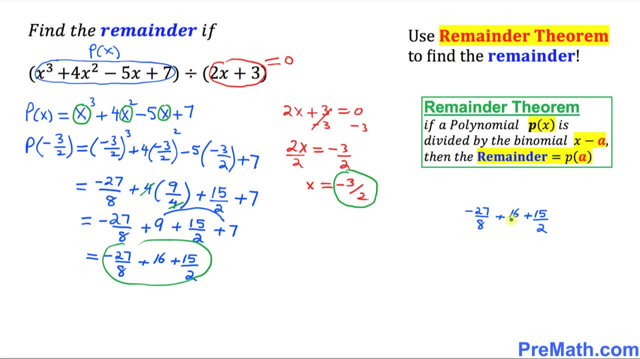 simplify it over here. As you can see, 16 could be written as 16 over 1 to make it a fraction, And we can see that our least common denominator, our LCM, is going to be 8.. So I can write this one negative. 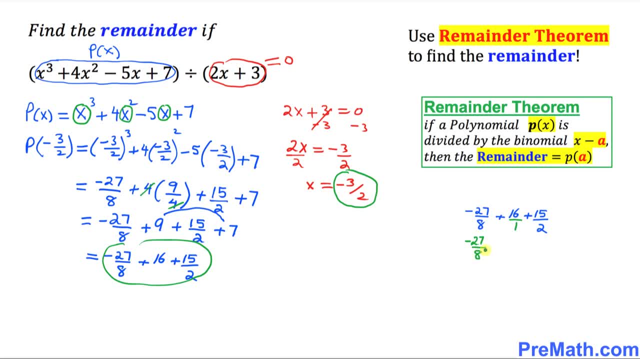 27 over 8.. If I multiply this one over here to make sure this is going to be 8 and 8 multiply, Okay. so here this is going to be 4 and 4.. So we are going to get plus 16 times 8 is. 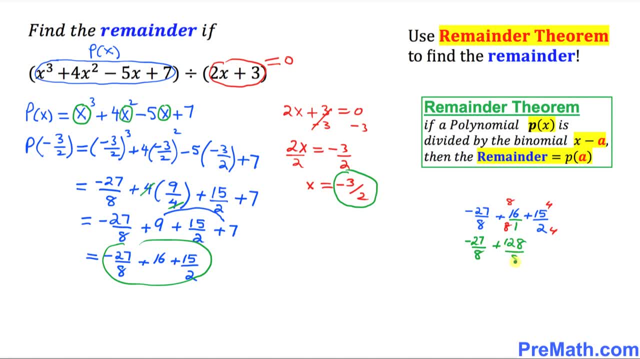 128.. 8 times 1 is 8.. Here, 60 divided by 2 and 5.. And do you notice that this, while this is less 1, the scale is getting bigger. So if you see we are going to get another value, 0. 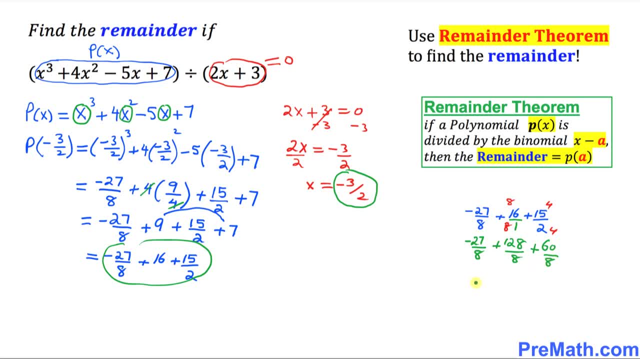 2 times 4 is 8.. Now we can see that we have the same denominator. Just put it once. You just write down negative 27 plus 128 plus 60. If you simplify the top part, that is going to give you 161. 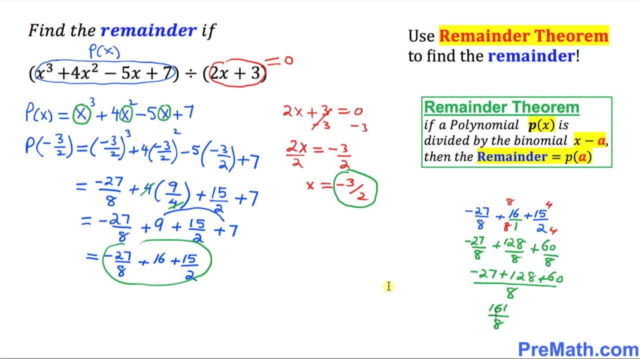 divided by 8.. So we are going to go ahead and put down this one over here. So p of negative 3 over 2 turns out to be 161 divided by 8.. And this 161 divided by 8 is our remainder. So that's our. 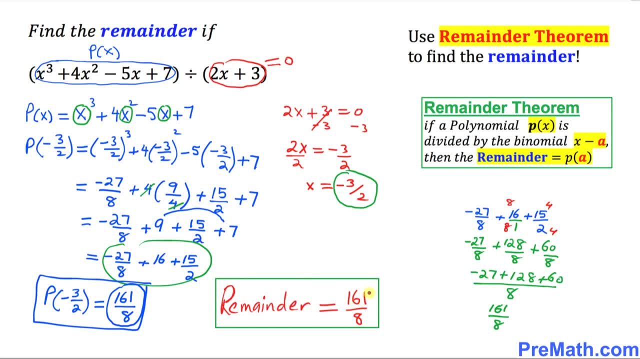 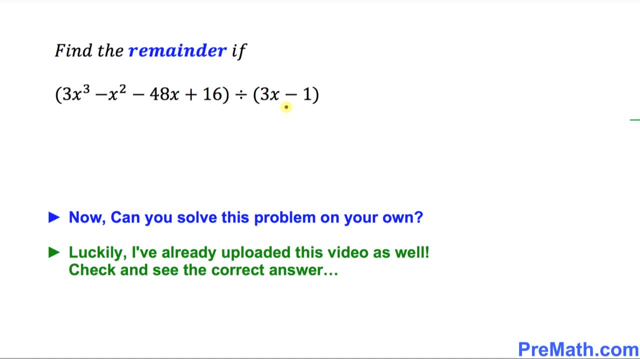 remainder. The remainder turns out to be a 161 divided by 8.. And that is our answer. And here is your assignment. Can you do this problem on your own? now You can take your time. You can pause the video. Luckily, I have already uploaded this video as well. Please go ahead and check it out and see the correct answer. Thanks for watching And please don't forget to subscribe to my channel for more exciting videos. Bye.